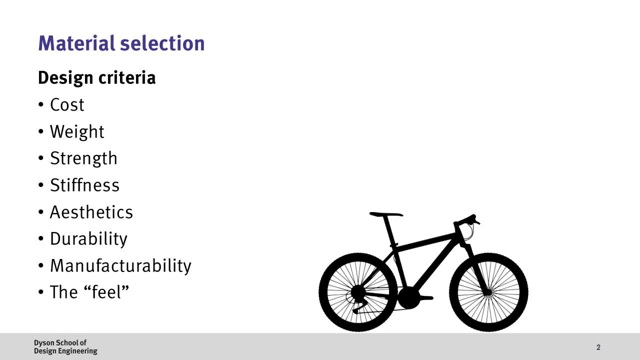 When designing a bike, we might first think about the design criteria, or what people care about. This can include things like cost, weight, strength, stiffness, aesthetics, durability, manufacturability and more abstract factors such as the feel of the bike. Then, if we think about what materials are available to us, there's an even greater list. 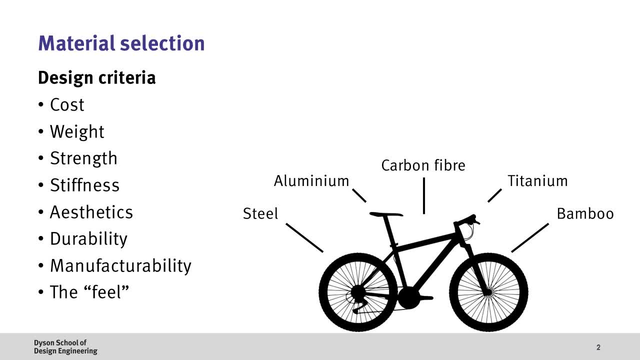 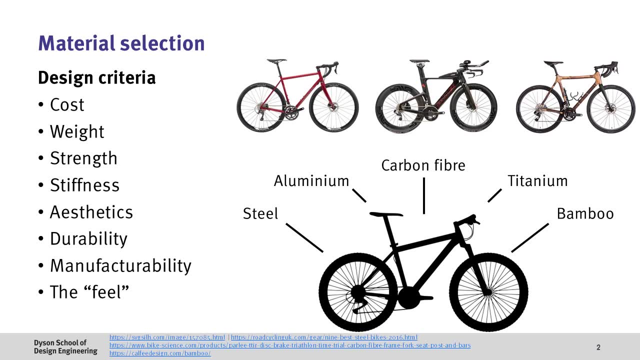 of possibilities, ranging from metals such as steel to composites such as carbon fibre, reinforced polymers and even natural materials such as bamboo. If we have a look at the market, we can see that there's a diversity of bikes available Out there which already use a whole range of these materials. Therefore, the question is which? 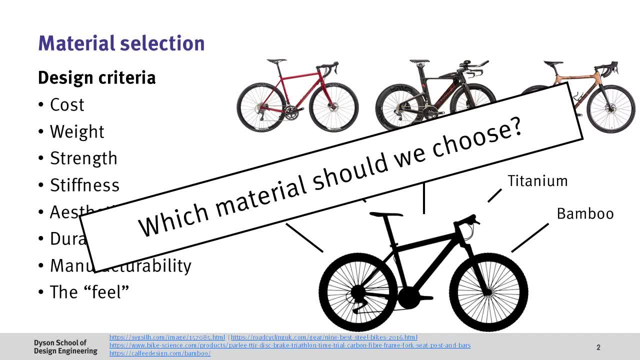 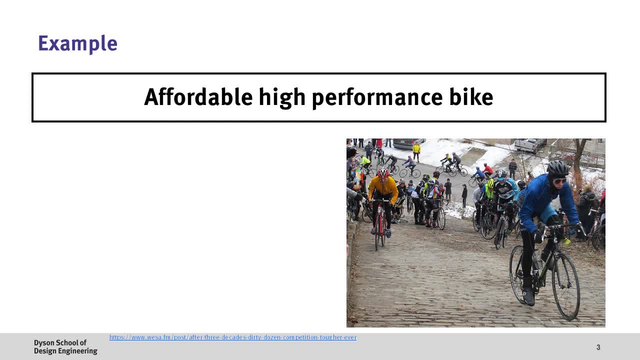 material should we use and are there any design tools which help us to make these decisions, To solve this problem? let's look at an example. Let's say you're a passionate cycler- not quite a professional, but proficient nonetheless. You're looking for a new bike. 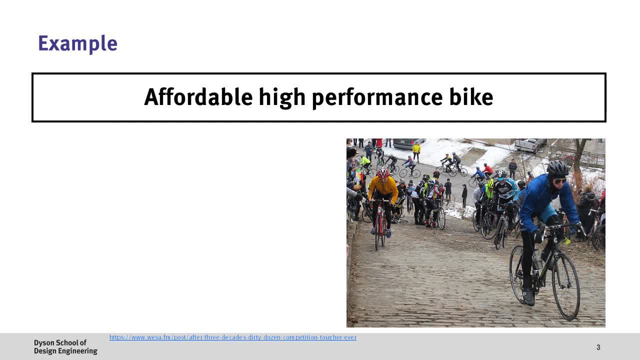 but you can't find the right one that's perfect for you, so you decide to make your own, which is high performance but also affordable. If we first think about what we care about or our design criteria, there are three main things. Firstly, weight. we want to do some hill climbs, and having a lighter bike will help with this. 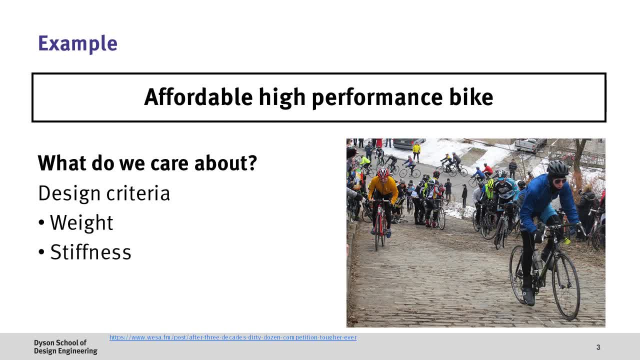 Secondly, stiffness. we want to transmit the power in our legs to the bike in the most efficient way and we don't want the frame bending And finally cost. we want a nice bike, but at the same time you want to make it affordable. If we then start to analyse the structure of the bike, we can see that there are three main things. 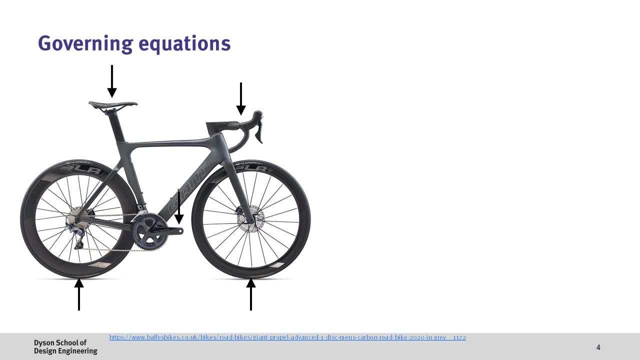 If we first think about what we care about or our design criteria, there are three main things. If we start to analyse the stresses that are found on a typical bike, the problem starts to become quite complicated. Therefore, in the initial design stage we want to simplify the problem as much as possible. 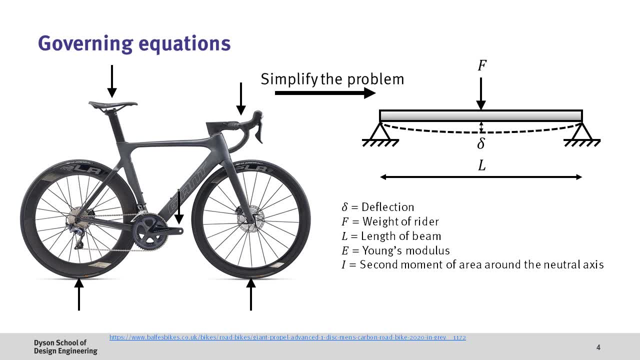 Here we've assumed a cylindrical rod of length L which is held at both ends. A force F, which represents the rider, is applied at the centre of the beam, which causes a deflection delta. Now, if we look up the mechanics equations related to this problem, 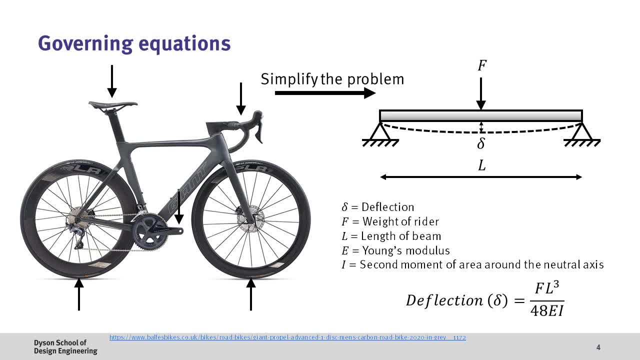 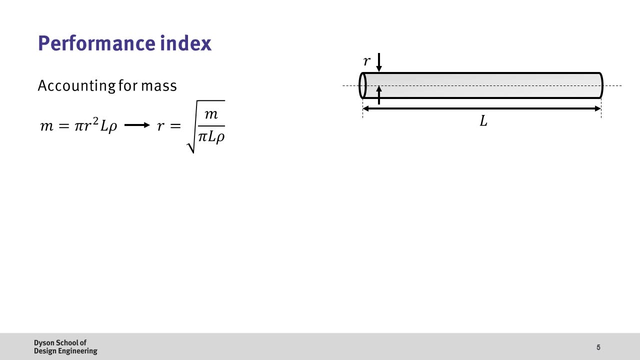 we can see that the central deflection can be given by F, L cubed over 48, E, I, where E is the young's modulus and I is the second moment of area. Next, if we then consider the mass of our cylindrical rod, we can define this as pi R squared, which is the area times by the length, to give the volume. 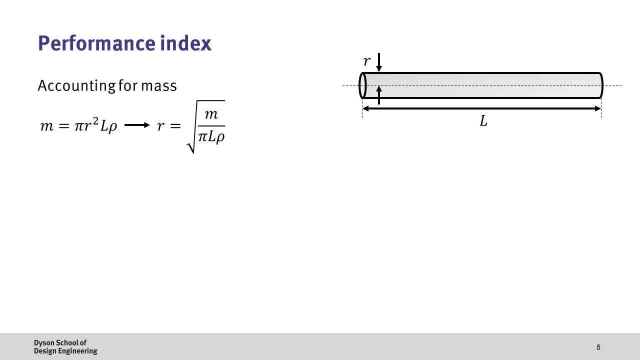 times by the density rho to give the mass. We can then rearrange this equation to make R the subject. Then if we bring back in the deflection equation and then substitute in the moment of inertia for a circle which is given as pi R to the 4 over 4, we come to a combined form of the equation. 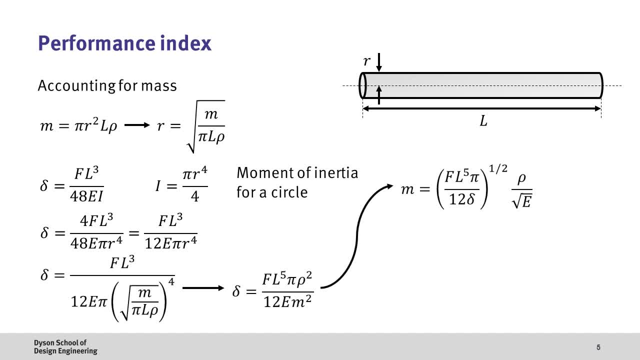 We can then substitute in the equation for R into the deflection equation, simplify and then rearrange for the mass. If we have a look at the various terms in the mass equation, we can separate these into two types. Firstly, there is a set of geometric and load parameters which are governed by the design of 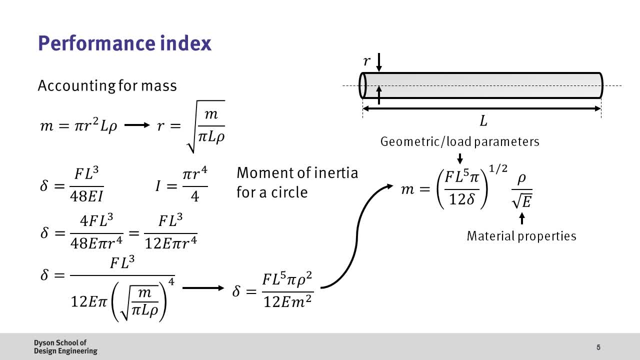 the bike. Secondly, and more importantly, we have properties which are defined by what materials we select. If we then take these material parameters and think about what we are trying to achieve, we would like to reduce the mass and therefore having a load value of rho over square. 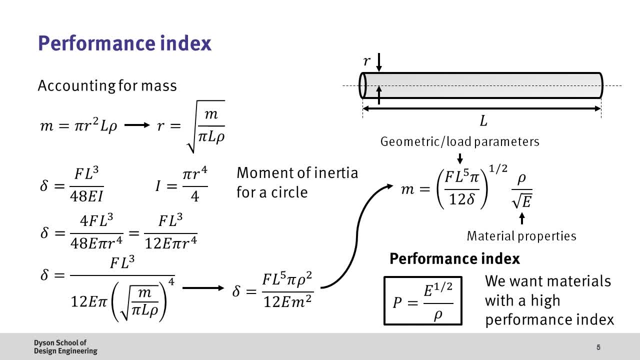 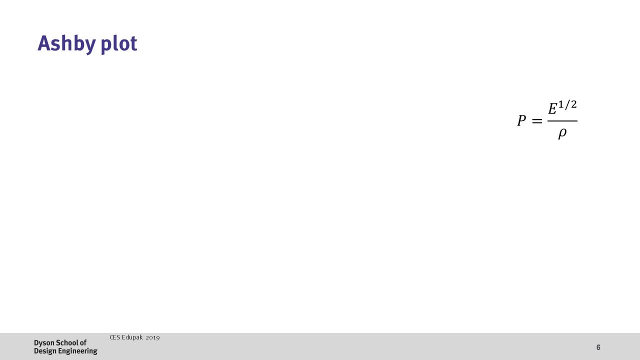 root E would achieve this Conventionally. we want to define a performance index which we maximise, So what we will do here is flip the equation. Let's flip this upside down to give our final performance index p, which is equal to square root E over rho. Ok, so now we have our performance index, which we define as square root E over rho. 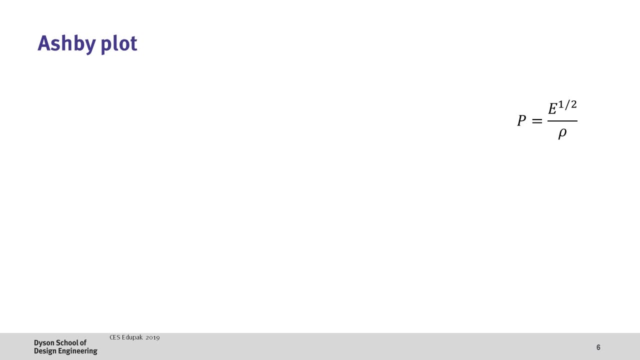 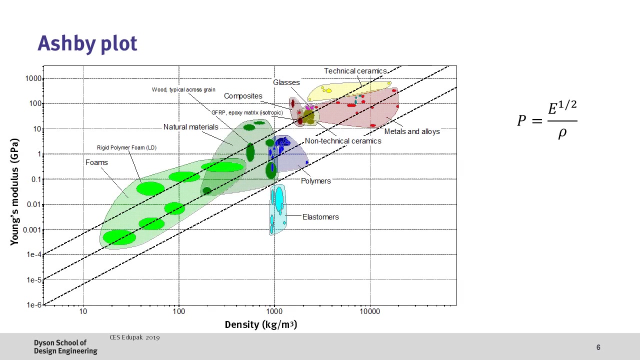 which we want to maximise. But how do we use it to help us select a suitable material for our bike? Firstly, let's consider an Ashby plot, which is a visual way of plotting two material properties against each other, In the case you see here. 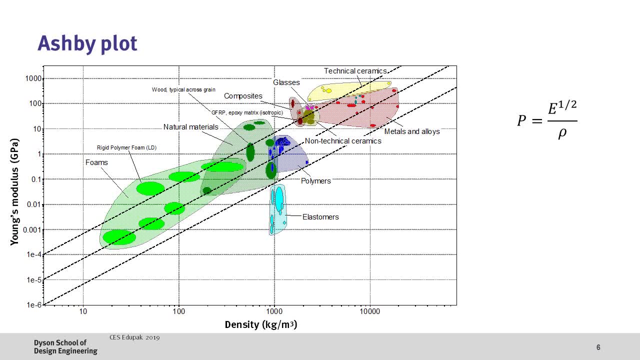 we have log of the Jung's equation. We have the density of the material, which is the stiffness of the material, And on the x axis we have the density Also labelled. here are a few material families, such as foams, polymers, metals and composites, as well as a few selected materials from these families. 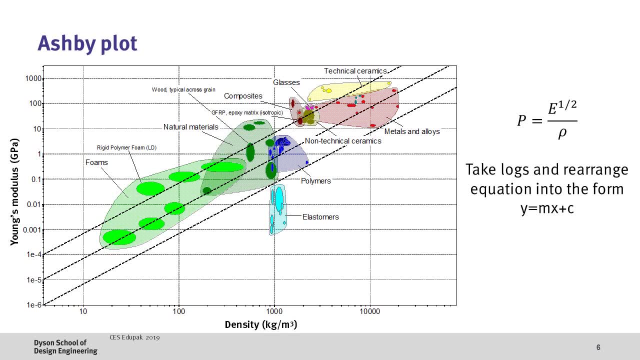 Now, if we return back to our performance index equation and rearrange this, we can start to down select materials for our application. If we take logs of both sides of our performance index equation and rearrange this into the form y equals mx plus c, we get the equation below: 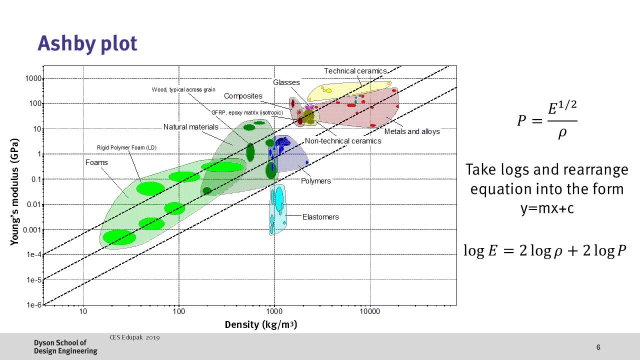 Now what this tells us is: if I draw a line with a gradient of 2 on my log-Jungs modulus against log density plot, all the materials along the line will have the same stiffness performance index. To get materials with a superior performance index, we need to move. 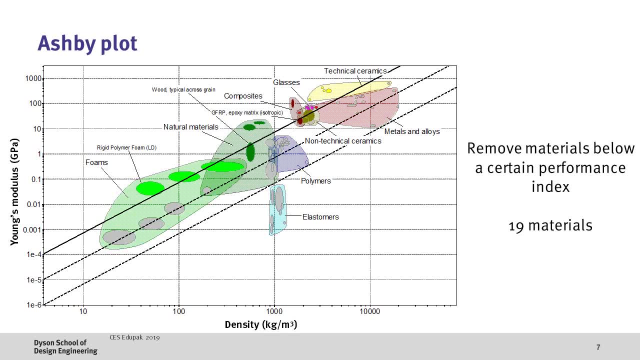 our line up to have a higher y intercept. So if we take that principle and from the free design lines shown in the Ashby plot select only materials above the top line, we can reduce the initial 69 materials to 19.. In doing this we've eliminated all elastomers and polymers. 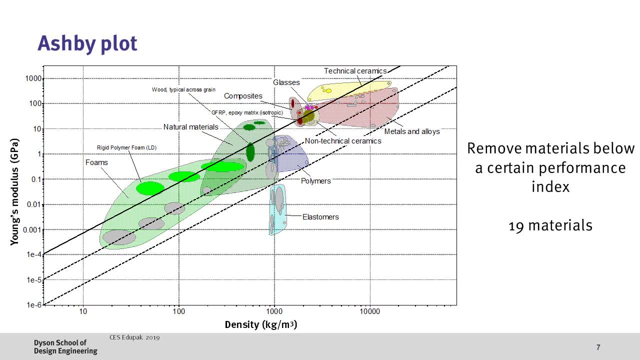 from the selection. This makes sense, since these materials generally have a low stiffness for a given mass. However, you can see that some materials with a very low Young's modulus are still in the analysis, such as foams. This is because, even though these materials, 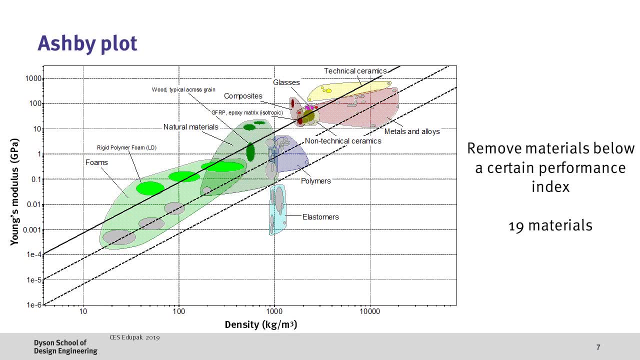 are very flexible. their densities are very low, which gives them a very good specific stiffness. However, in practice, it's unlikely you'd want to make a foam bike, as you'd need an impractical amount of material. So, in order to further filter the materials towards a practical selection, let's return. 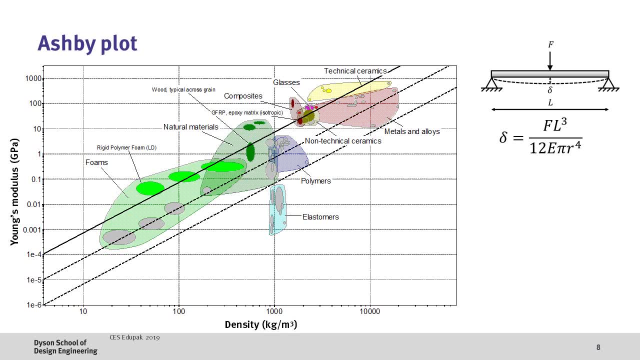 back to our original governing equations. In the original example, where we simplified the problem to a beam supported on either end with a centrally loaded force, we can define the deflection as a function of the geometry force and Young's modulus. If we 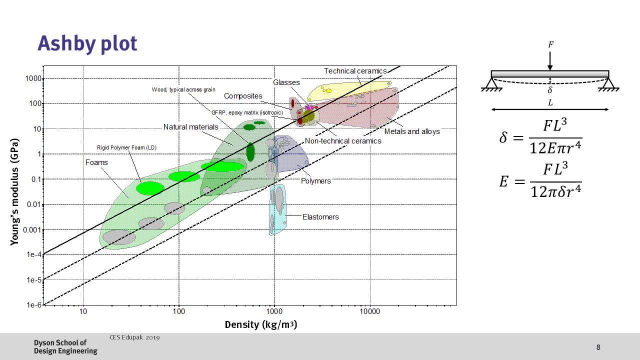 then rearrange this equation. we can make the Young's modulus the subject. Then we can put some assumptions into our analysis. For example, let's assume that the maximum force is 1000N, the length of the beam is 90cm, the radius is 4cm and the maximum 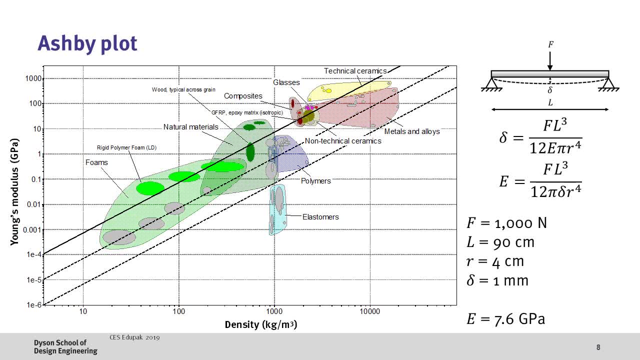 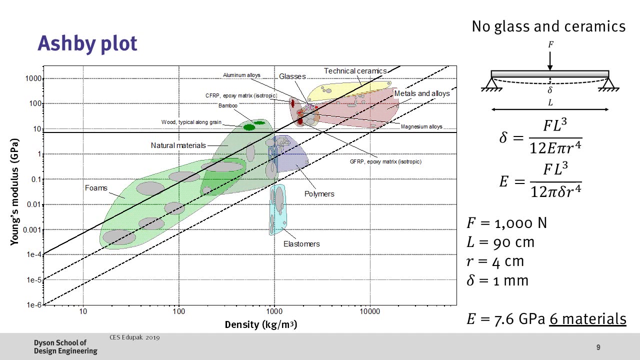 allowable deflection is 1mm. If we put these numbers into the equation, we can get a lower limit for our Young's modulus, which is 7.6 GPa. Finally, if we eliminate glasses and ceramics from our analysis, we get to 6 remaining materials. 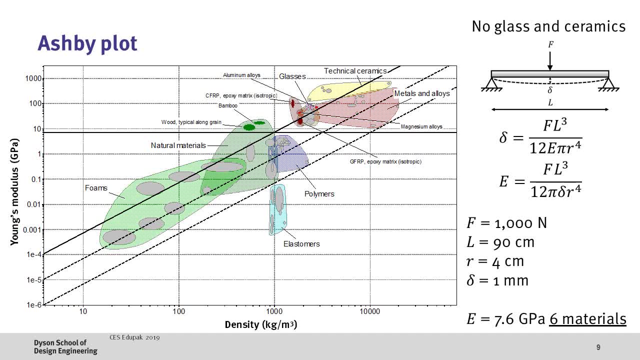 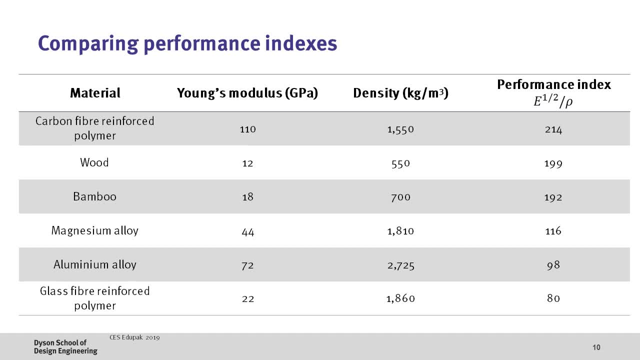 which is much more manageable to do an in-depth analysis. So if we now take our 6 remaining materials, their Young's modulus and their density, we can calculate their stiffness performance index and rank them. Here it can be seen that carbon. 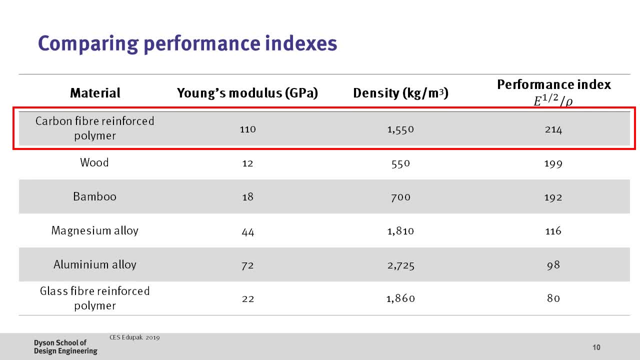 fibre reinforced polymers rank the highest with natural materials such as wood and bamboo, surprisingly following and ahead of materials such as magnesium and aluminium alloys, as well as glass fibre reinforced polymers. This is already really useful. however, it's not the whole picture. 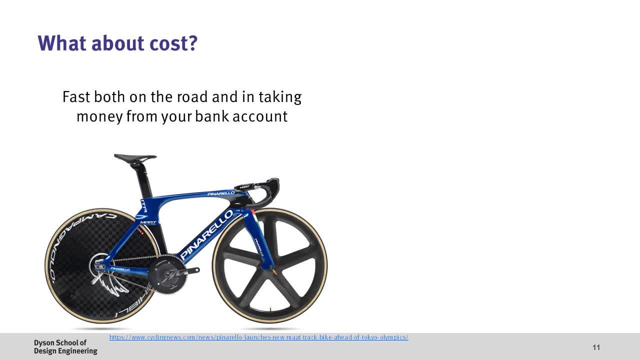 So earlier, our design objective was to make an affordable, high performance bike, and whilst carbon fibre composites are very fast on the road, they're equally fast in taking money from your bank account. Therefore, we need a way of factoring in the cost of the material. 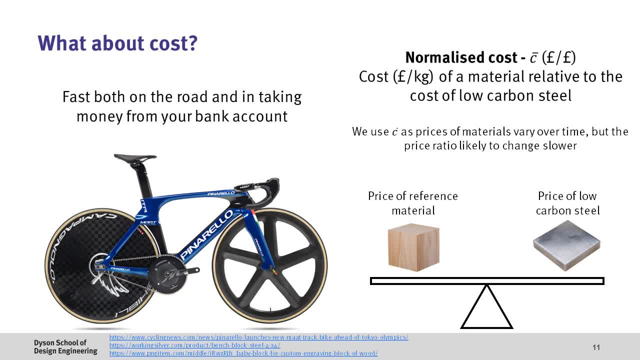 Now, whilst we could just incorporate the cost of materials into a new performance index, it's often better to use normalised cost of a material relative to low carbon steel. The rationale for this is that material prices fluctuate over time and therefore the optimal 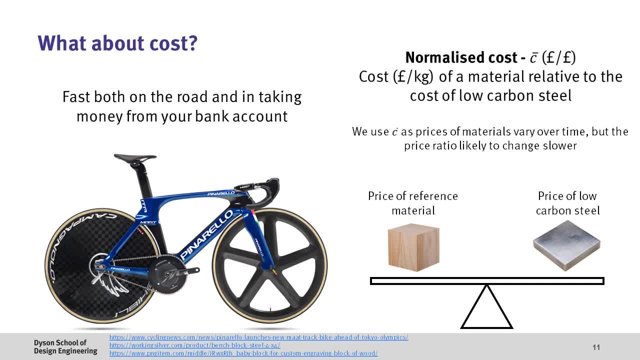 solution will depend on when you do the analysis. However, the relative cost of materials in theory varies less than their absolute values. Thus, taking the normalised cost of a material relative to low carbon steel, which has a very stable price, can give us much more consistent answers. 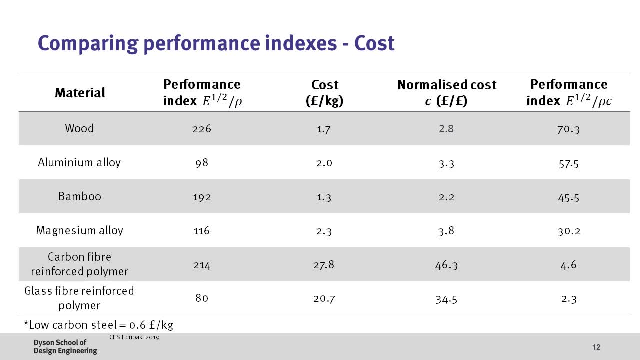 Now, if we then take the performance index of our six materials and incorporate the normalised cost into the performance index, we can re-rank them. In this case, we put the normalised cost as the denominator, as a lower cost would increase. 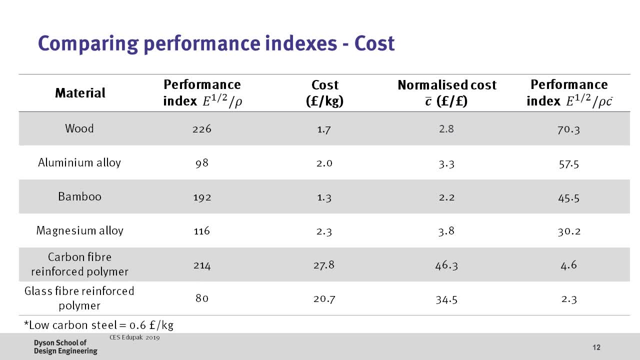 the performance index. Also, we've arbitrarily put a unity weighting on the performance index. here We can class this as the performance index. Also, we've arbitrarily put a unity weighting the cost performance index. but if this was more or less important, this would obviously 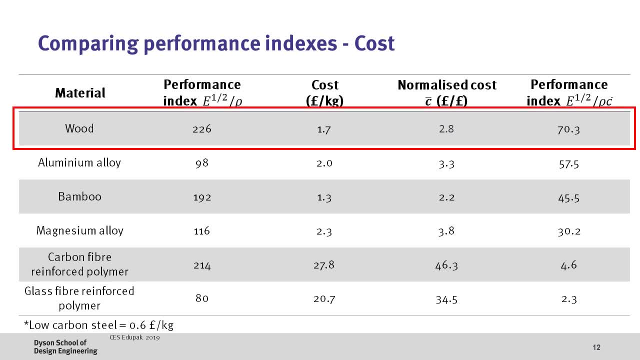 change the eventual answer Now. after factoring in costs, we can see that wood, aluminium alloys and bamboo are the top materials with carbon fibre, second to last. now, Therefore, does this mean that we should all make wooden bikes? Invariably, the answer is no. 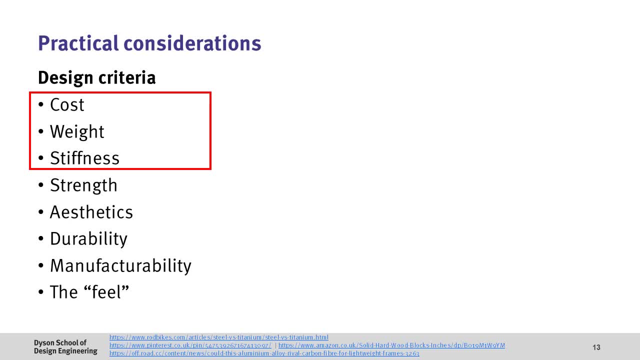 If we look back at our initial design criteria, this included a long list of factors and in this analysis we only consider the cost, weight and stiffness. One could repeat the analysis to look at the strength of the material and we would come to a slightly different answer. 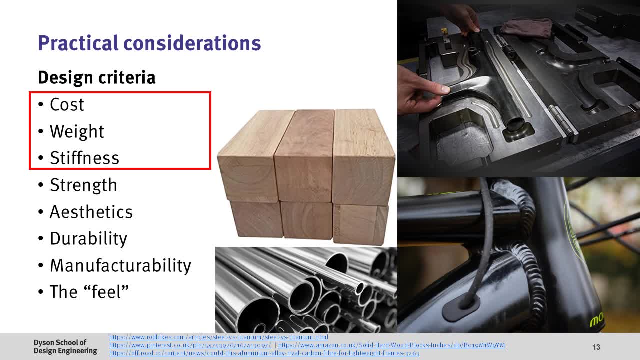 However, one of the more difficult factors to account for in these performance indices is often the manufacturability, which also affects the overall cost. Whilst we have factored in costs from a materials perspective, In this analysis we can see that wood, aluminium, alloys and bamboo are the top materials with 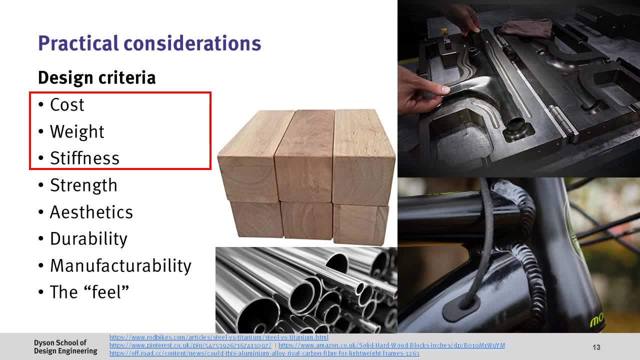 the highest performance index. This does not include the cost of manufacturing the materials into the final form that we want. Wood, for example, which is highly ranked, would need to be cut into the desired shape, whereas metal can often be manufactured at low cost through an extrusion process. 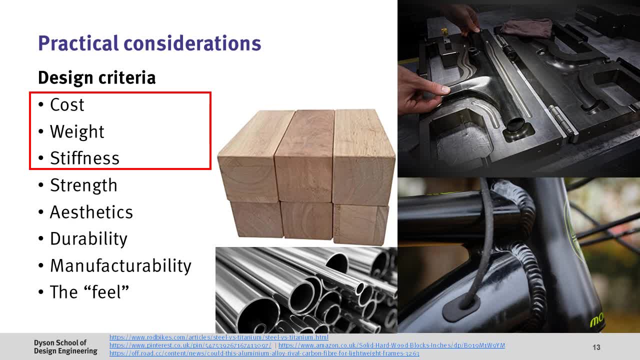 Assembling the frame is another complexity. Metals can often be welded or brazed together, but wood needs to be glued together, which requires longer setting times. Carbon fibre components require a mould And a lay-up process which is often very manual and requires costly tooling. 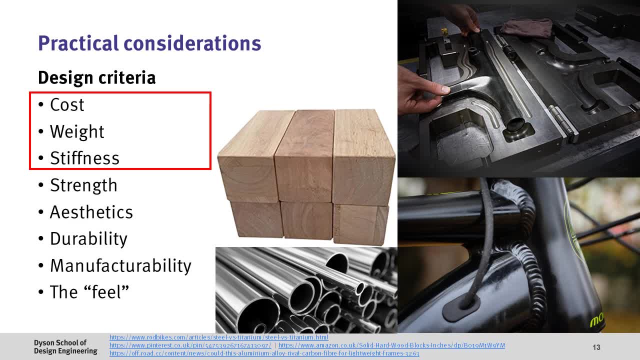 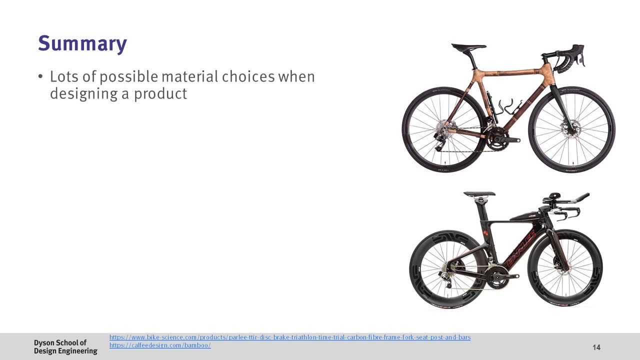 Therefore, whilst the Ashby plot and performance index analysis is useful, other factors, especially manufacturability, need to be factored in. This can, of course, be added as an additional filter in more advanced analysis, but hasn't been done here. So, to summarise, 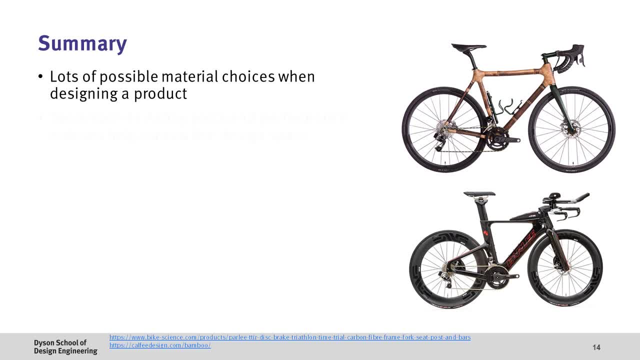 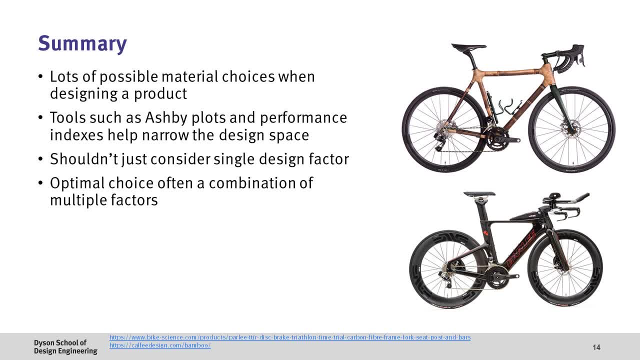 just consider a single design factor. An optimal choice is often a combination of multiple factors, And quantified analysis does help with decision making, but we need to consider the practical implementation of our designs with key factors such as manufacturability. So thank you very much for watching this video on material selection using Ashby plots and. 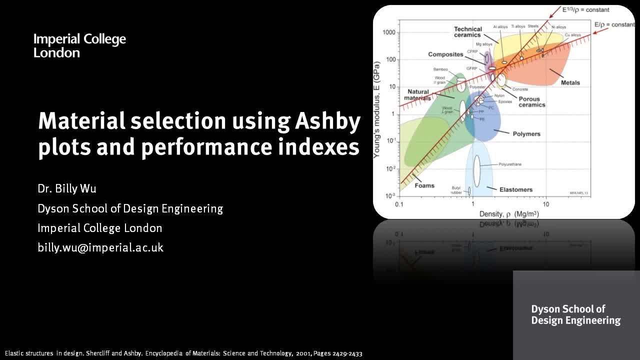 performance indices. Hopefully, this has provided you with some useful tools to help you with your future projects involving material selection.